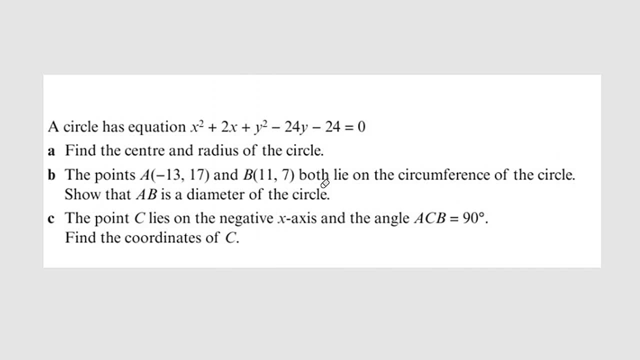 The points a and b with their corresponding coordinates. both lie on the circumference of the cycle. We are asked to show that the line segment a, b is a diameter of that cycle, And the last question here reads: The point c lies on the negative x axis and the angle. 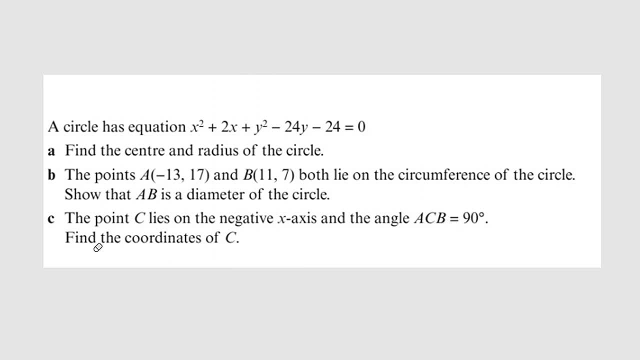 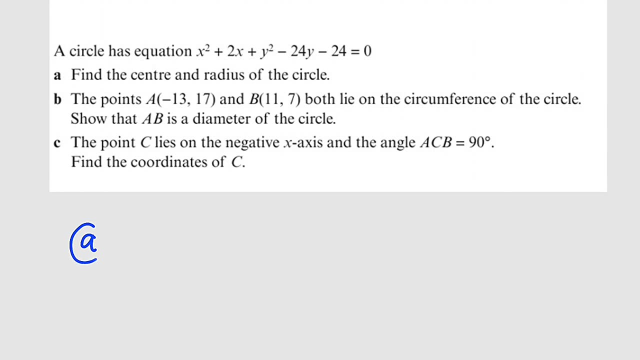 a, c, b is equal to 90 degrees. We are asked to find the coordinates of c. Alright, let's get started. Let's start with question a. We are asked to find the coordinates of the centre and the radius of that cycle. 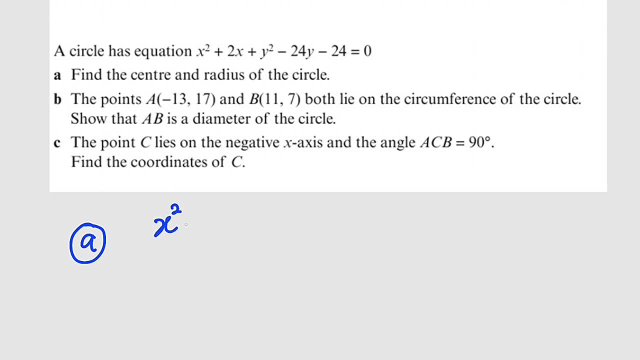 Let's start with question a. We are asked to find the coordinates of the centre and the radius of that cycle. The equation given to us is x squared plus 2x plus y squared minus 24y minus 24.. This is equal to 0.. This is an equation of a cycle in general form, which we can write as x squared. 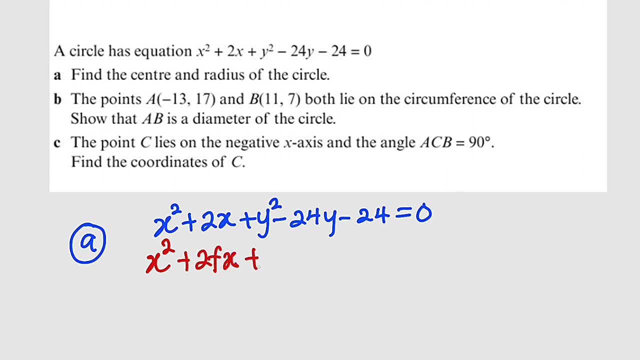 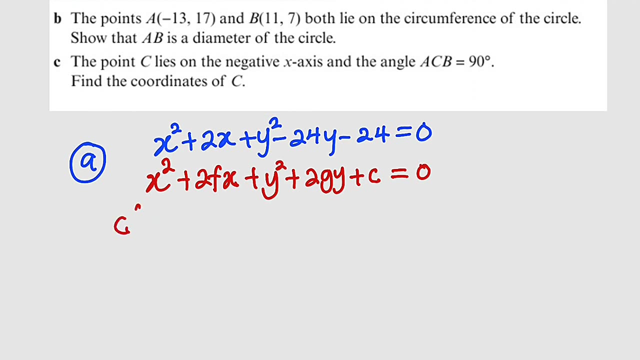 plus 2fx plus y, squared plus 2y, 2 g, y then plus c, the whole of this equal to zero, where the center of that cycle has the coordinates negative f, comma, negative g, if you can recall, and the radius of the cycle can be of 10. 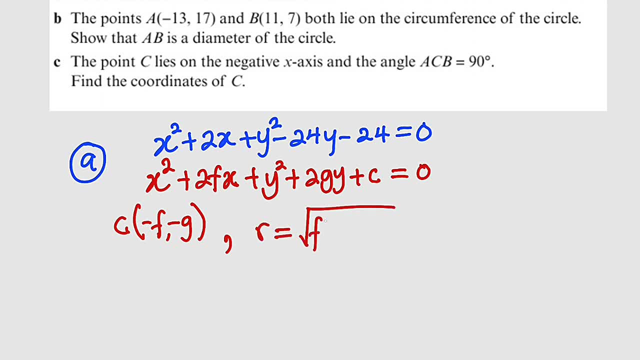 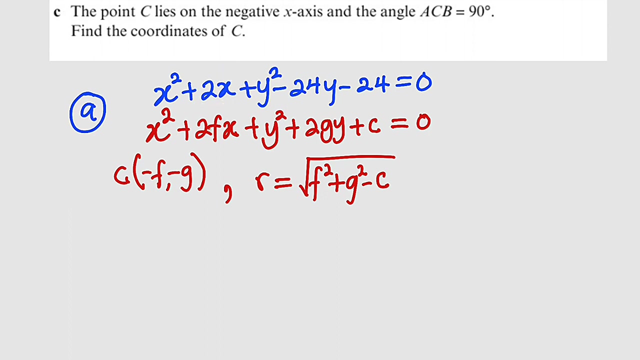 by taking the square root of f squared plus g squared minus c. so this is what we need in order to find the center of the cycle and the radius of that cycle. so let's bring out the data. let me start with f to find f from here. you can see: the coefficient of x is 2, while the coefficient of x 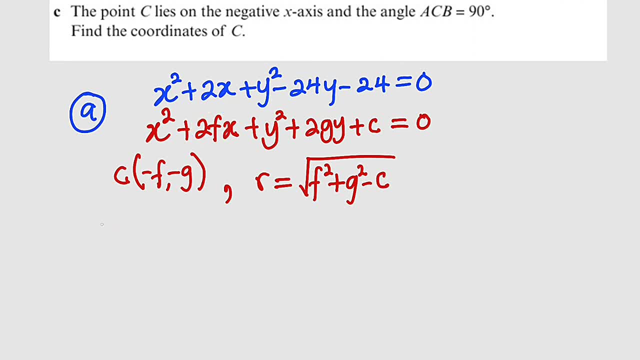 here is 2f, which means that 2f is equal to 2. if you divide both sides by 2, you have f to be equal to 1. then you need also to find the value of g. from here you can see the coefficient of y is negative 24, while the coefficient of y here is 2g. 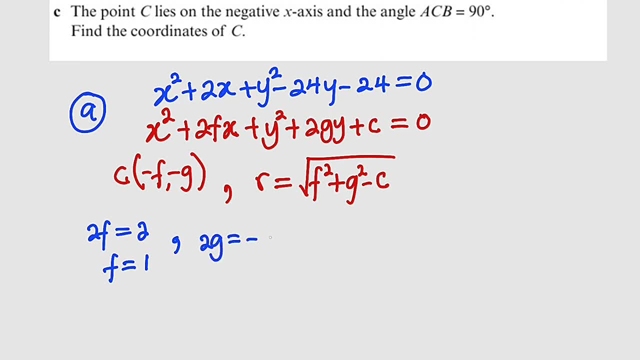 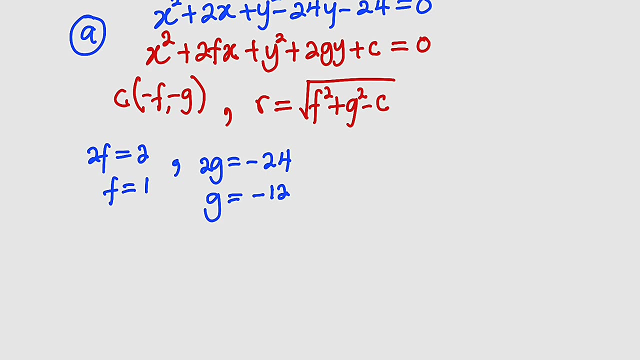 meaning that 2g is equal to what negative 24.. if you divide both sides by positive 2, you have g to be negative 12.. so what do we say? we say that the center of the cycle is given as negative f and negative g. 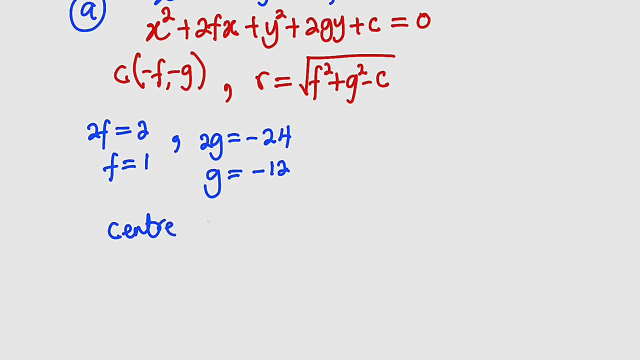 so the center of that cycle has the coordinates negative f. f is 1. if you negate it, you have negative 1. then g is negative 12. if you negate it, you have positive 12, and hence this is the center of that cycle. then, coming to the radius, the only thing we need to find out is that the center of the cycle is negative 12.. 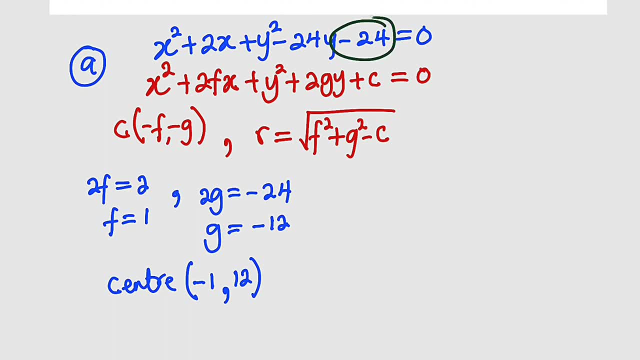 the only thing we need to find is c, which is the constant, and constant in this case is 24 negative, so we can clearly see that c is equal to negative 24.. already we have f and g, so all we have to do is to substitute them into this equation. 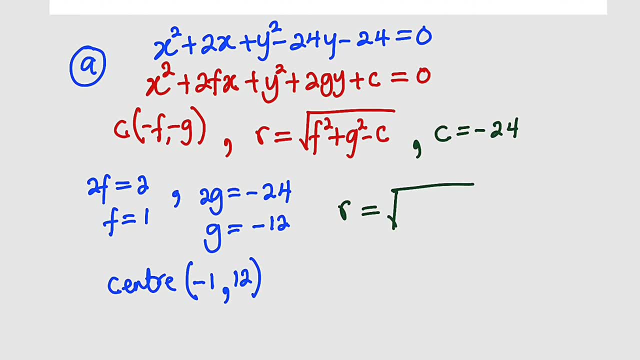 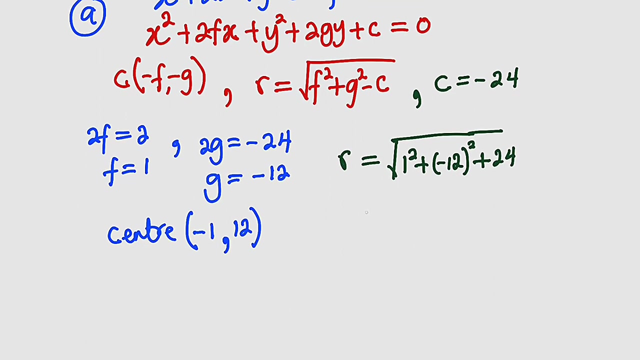 and hence our radius is equal to the square root of 1 squared. that is f squared, then plus g squared, which is what negative 12 squared, the minus c, c is already negative, so minus preservatives will bring it to positive 24. now let us simplify and get the radius. this is equal to the square. 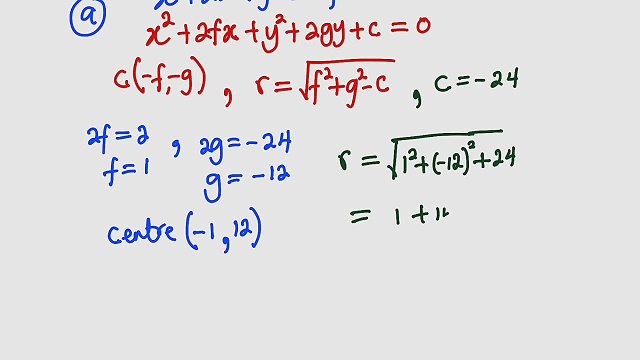 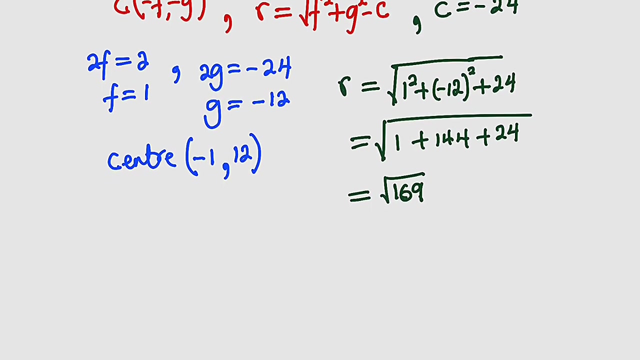 root of 1 squared is 1, plus negative 12 squared is 144. then, plus 24, 1 plus 144 will give us 145, plus 24 will give us 169. so this is the square root of 169, and square root of 169 is 13. hence the radius of that cycle is 13 units. so we have obtained the center of the. 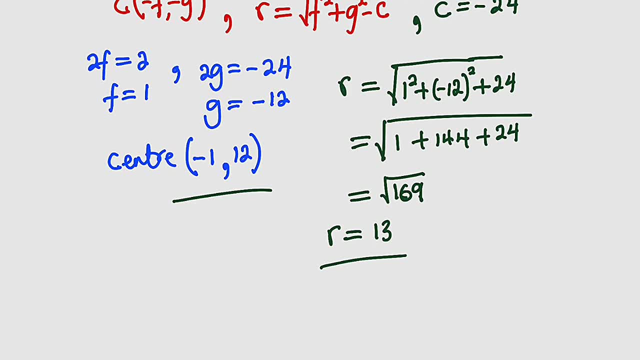 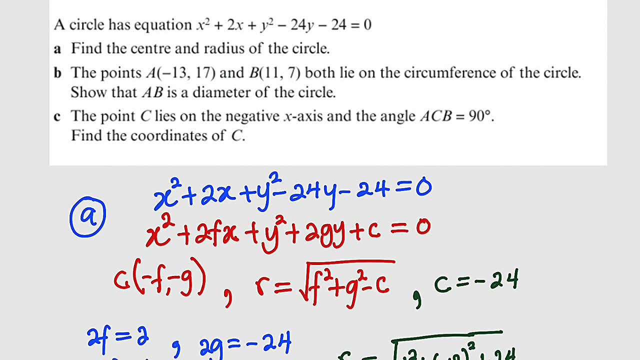 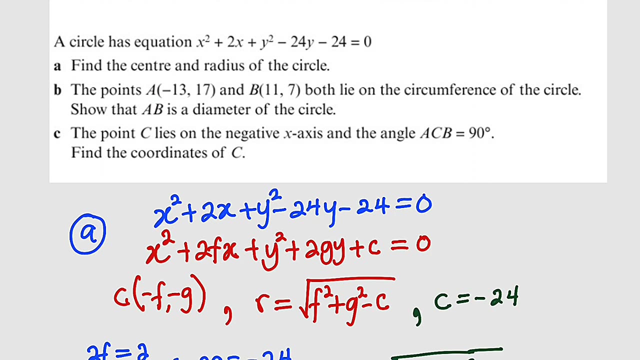 cycle and also the radius of that cycle. this is not the only way to do that. you can convert it into standard form, but we are not going to do that in this tutorial. then the second question, which is the b part. it stated that we have a point a b, which is a line segment that lie on 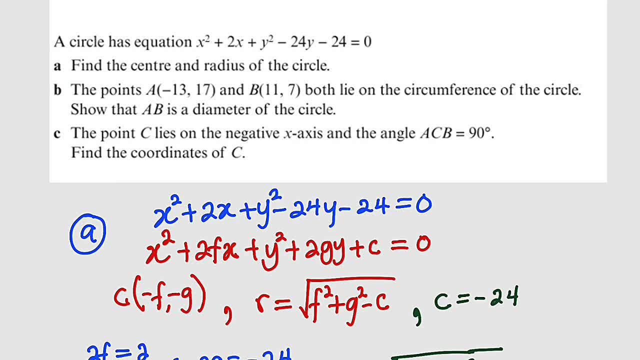 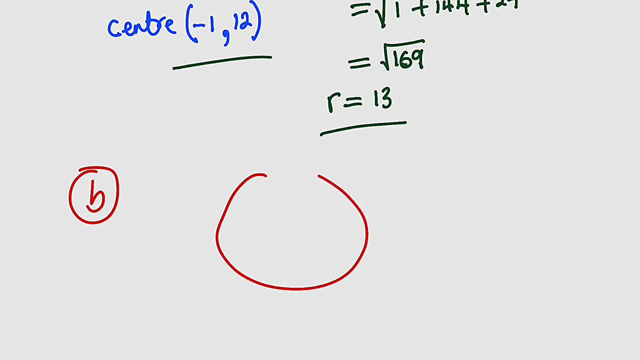 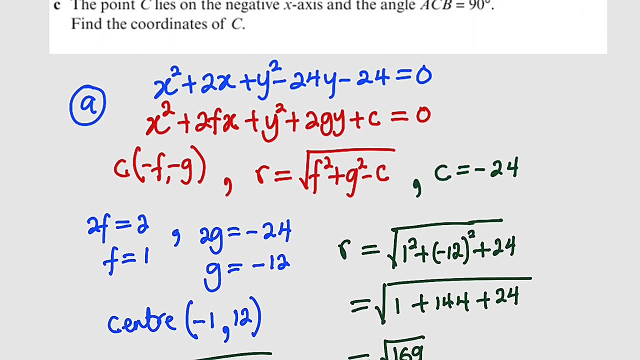 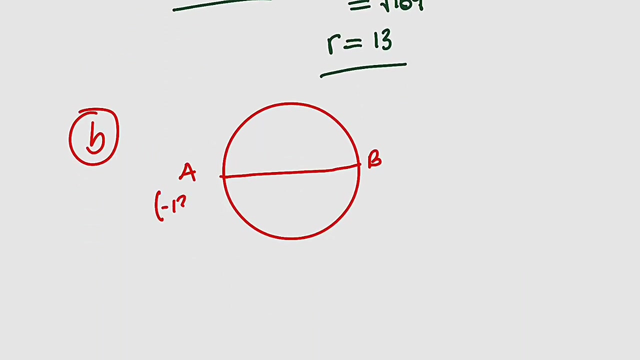 the circumference of that cycle. we are asked to show that a, b is a diameter. so now let us construct a cycle. so this is b. suppose we have a cycle like this and we have a line a, b. what are the coordinates? negative, 13, 17. negative 13, 17. then the b: we have 11, 7. we have 11. 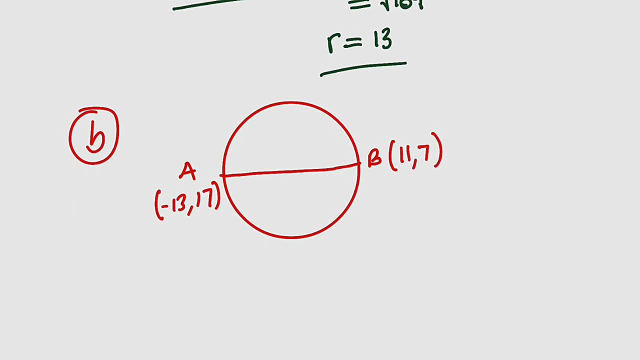 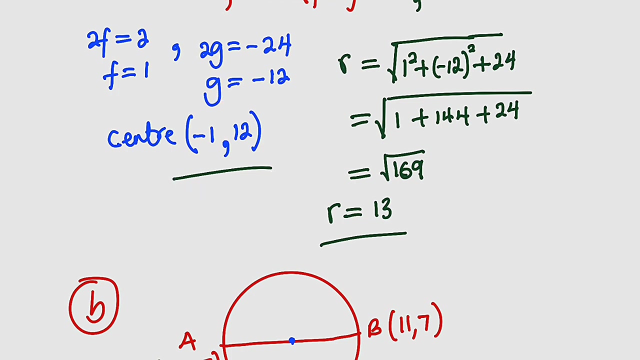 7. if line a, b is really the diameter of this cycle, then what will be the center of this cycle? we are going to take the midpoint. if the midpoint corresponds to the center of the cycle, which we have here as negative 1 comma 12, then we conclude that line AB is really a. 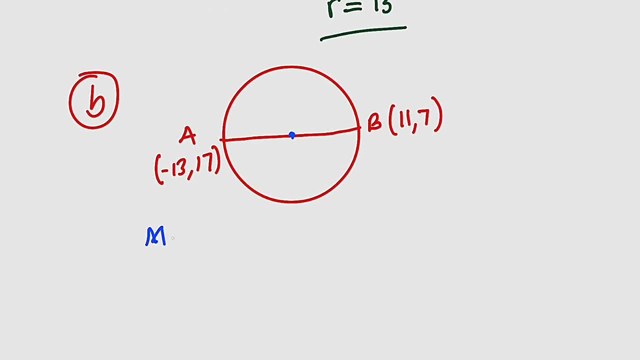 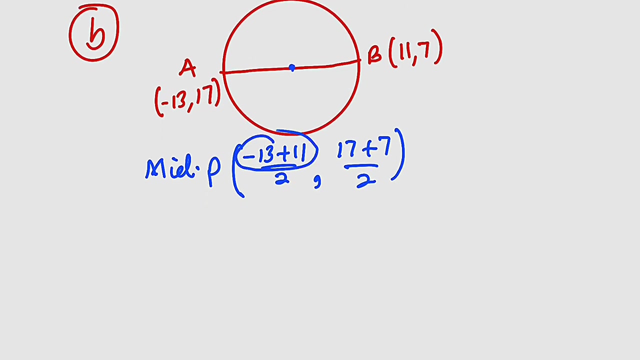 diameter. so let us take the midpoint. midpoint will be what you add the x axis, you divide by 2. negative 13 plus 11, you divide by 2, then you add the wise 17 plus 7, you also divide by 2, so negative 13 plus 11 will give us negative 2 and 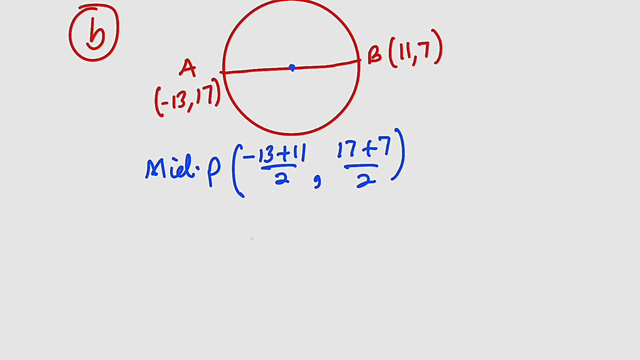 negative 2 divided by 2 is negative 1, so we have negative 1 for X. then if you add this together- 17 and 7- you get 24. divided by 2 is 12, and hence this is the midpoint of the line, segment AB, which should correspond to the center of that. 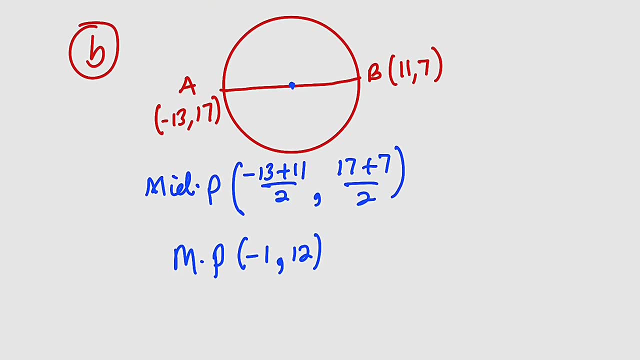 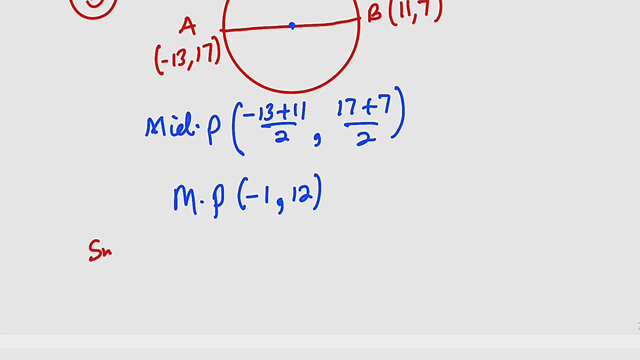 cycle which we have here. you can see, they're exactly the same. you can see they're exactly the same and you can see they're exactly the same, and hence we say that line AB is really the diameter of that cycle. so how can we conclude? we can see that, since midpoint is equal to the center, hence AB is a. 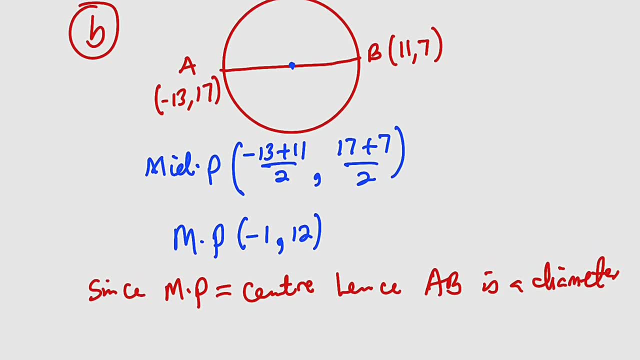 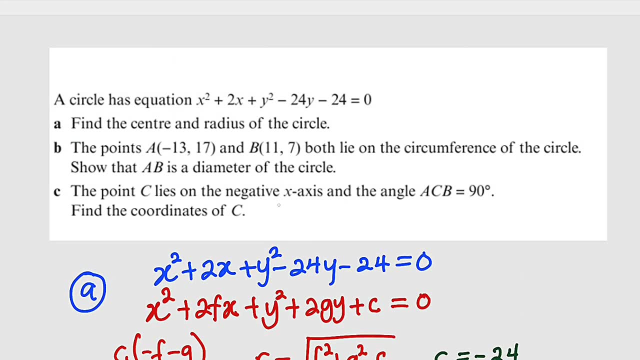 diameter. right, so we are done with this question. now let us move to the next one, which is the last one, the point C, which is the last one. the point C lies on the negative x-axis and the angle ACB lies on the negative x-axis and the angle ACB. 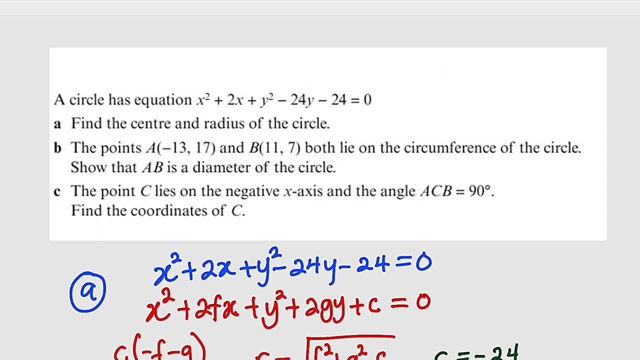 lies on the negative x-axis and the angle ACB is equal to 90 degrees. we have to is equal to 90 degrees. we have to is equal to 90 degrees. we have to find the coordinates of C all right. find the coordinates of C, all right. 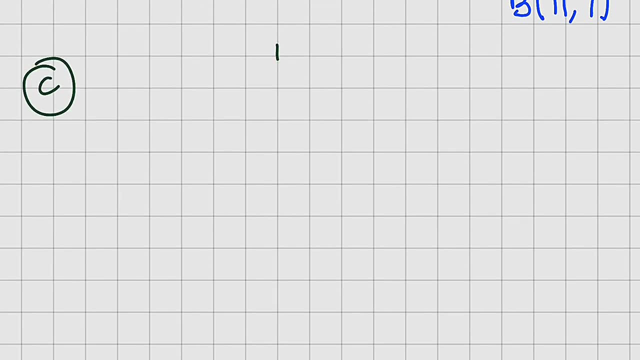 find the coordinates of C. all right, this is our C part. suppose we have Y. this is our C part. suppose we have Y. this is our C part. suppose we have Y axis here. we have X axis here. suppose we axis here. we have X axis here, suppose we. 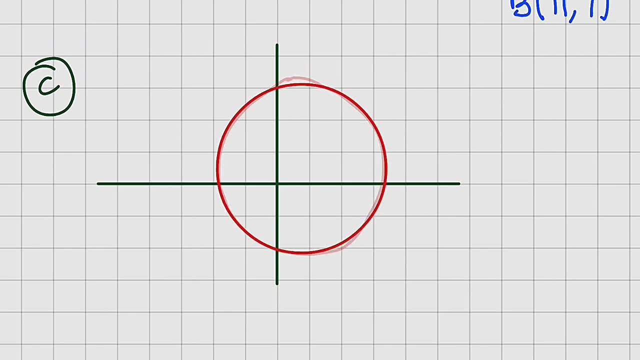 axis here we have X axis. here. suppose we have a cycle, simple cycle like this. let have a cycle, simple cycle like this. let have a cycle, simple cycle like this. let us add the two points given to us, which us add the two points given to us, which. 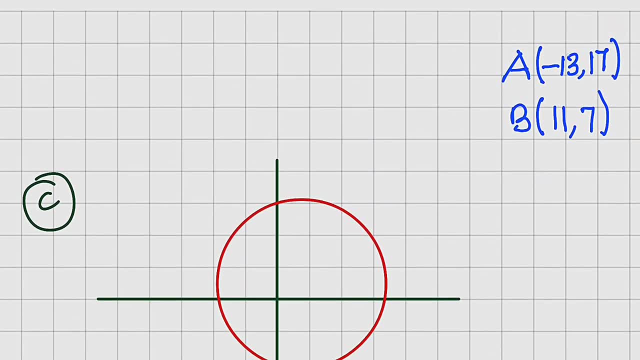 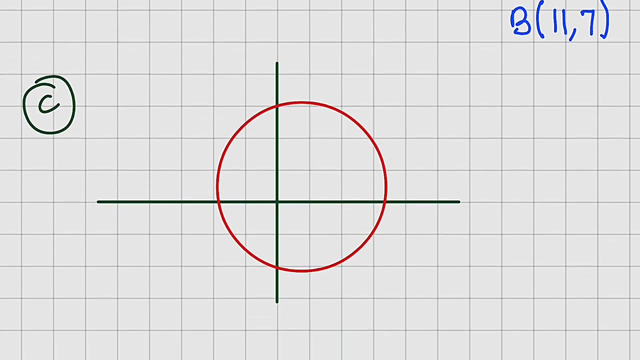 are a, b already. i have them here. so x is negative, y is positive, which is in the second quadrant here, and the coordinates of b are all positive, which means it lies in the first quadrant. so let us place them here, so we may have something like this: so suppose we have a point a here and 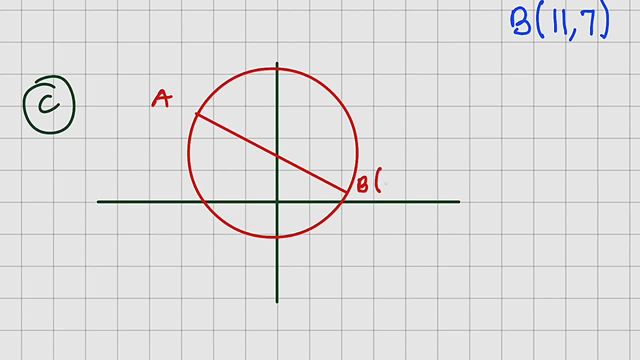 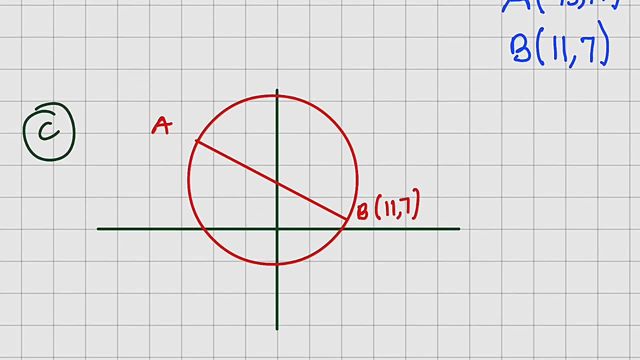 a, point b. here the coordinates of b are 11- 7 and point a has the coordinates negative 13- 17, so this is negative 13, 17.. according to the question, there is another point, which is c, that lies exactly on x negative axis. this is x axis and this is x axis, but this is negative. 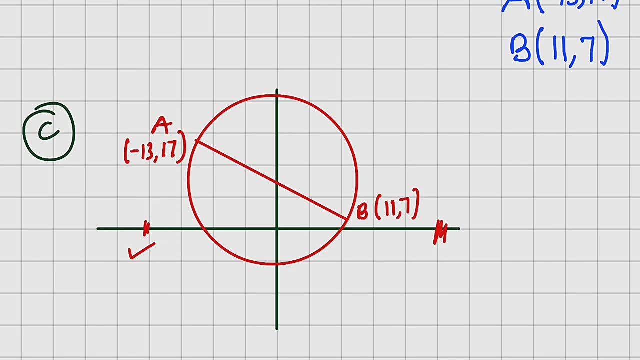 while this is positive. so it means this leg exactly. so let us sketch it from a exactly onto x axis and from b down to that same axis, and we form a right angle here, which is angle 90 degrees. so we have point c. what you should know about this point c is that the y coordinate at that point must be equal to zero, because it 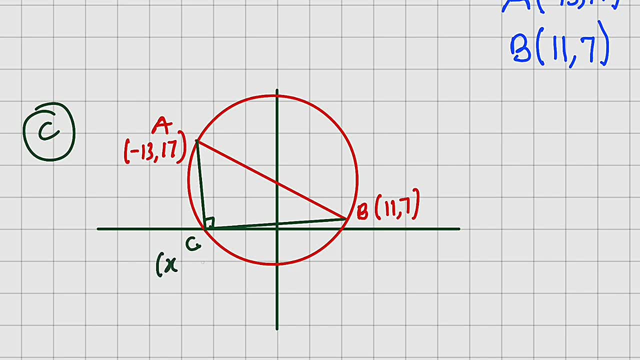 lies on x axis. so we have x, which we don't know, but y coordinate must be zero, all right. and another thing you should remember is that this line ac and cb are perpendicular to each other. i remember that the slope of two perpendicular lines are always the 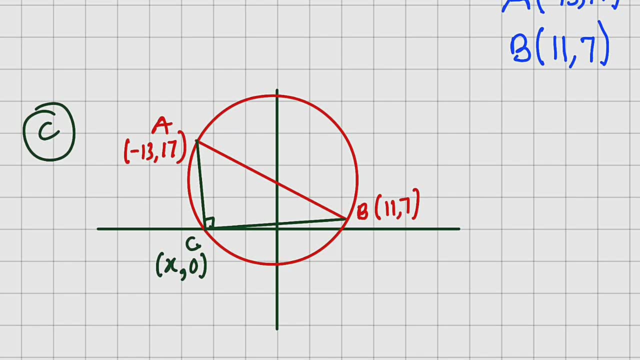 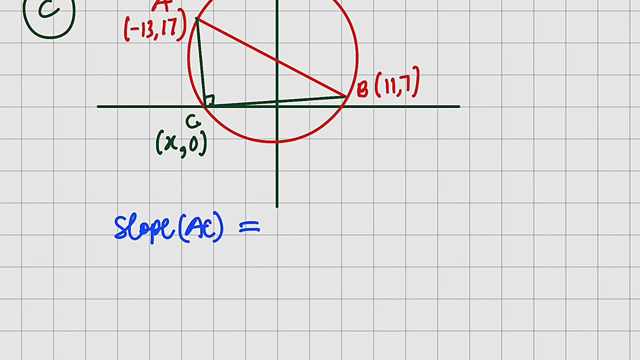 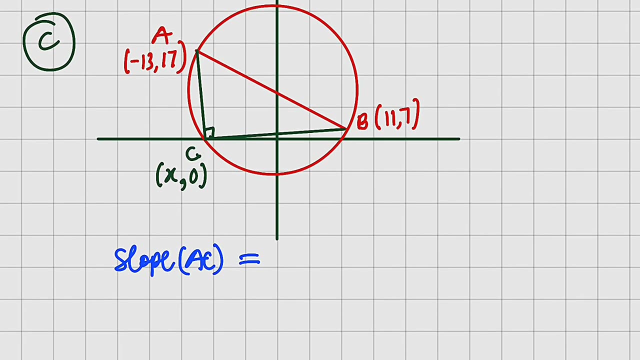 negative reciprocal of each other. so now let us find the slope of line ac. so we have slope of line ac which is equal to y2 minus y1 divided by x2 minus x1. and you can always start from other lines. let me start from a y coordinate at that point is 17 minus y, here is 0, so we have minus 0. 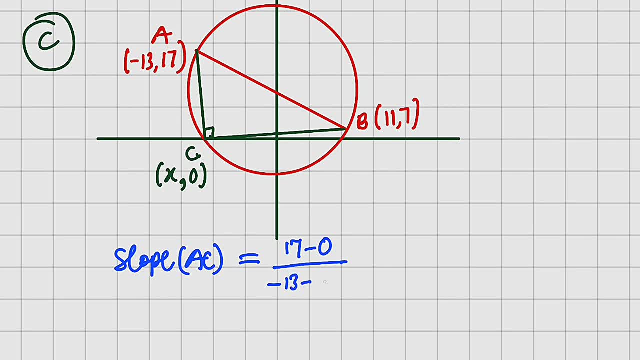 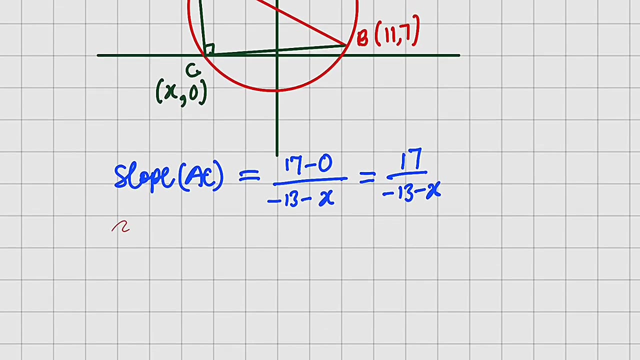 divided by x negative 13, then minus another x. here, if you simplify this, you have 17 divided by negative 13 minus x. this is the slope of line ac. now what about bc? slope of bc? the same thing. y here is 7, so we have 7 minus y. here is 0 minus 0 divided by 11 minus x. 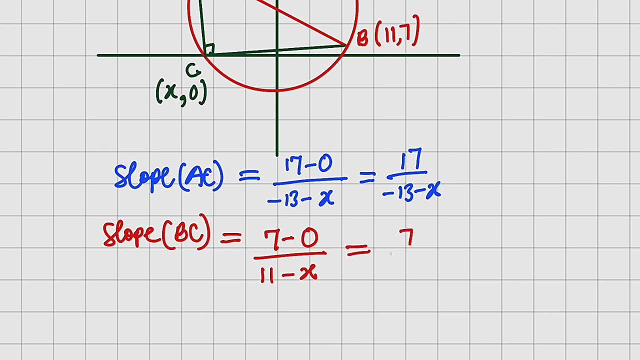 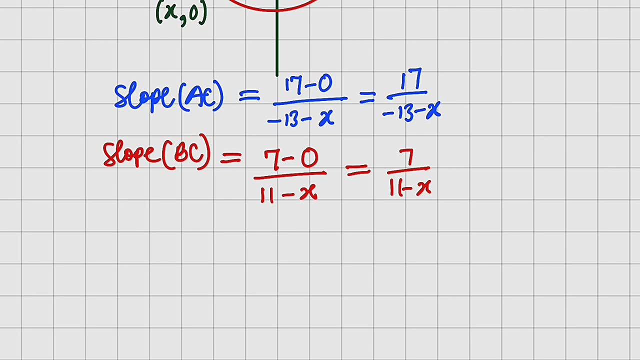 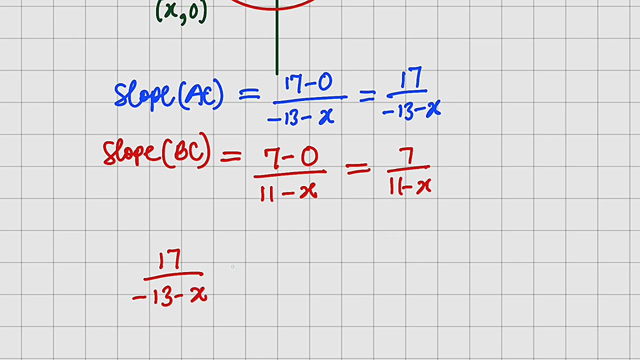 simplify, and of 10, 7 divided by 11 minus x. but i told you, the two slopes are negative, reciprocal of each other, which means that this 17 divided by negative- 13 minus x- is equal to negative, the whole of this 11 minus x. 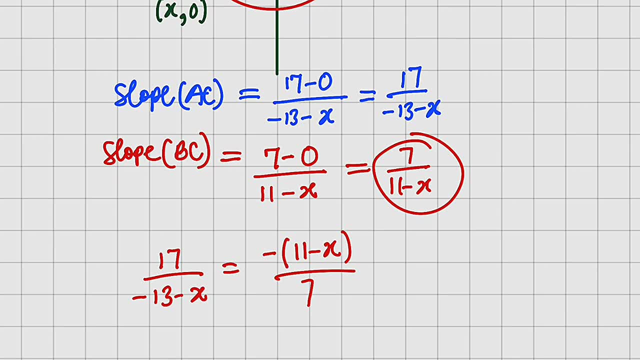 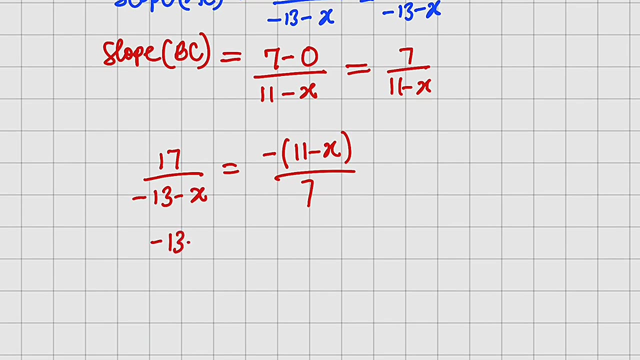 divided by seven. all you have to do is to take the reciprocal of this by flipping upside down the nominator and numerator. then you negate it by multiplying by negative sign. so this is the equation we need to solve for x. by cross multiplication we have negative 13 minus x. 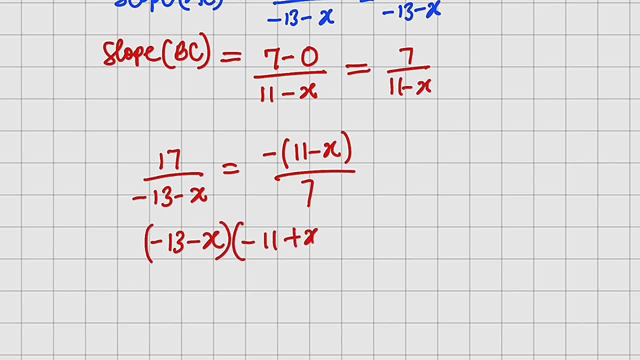 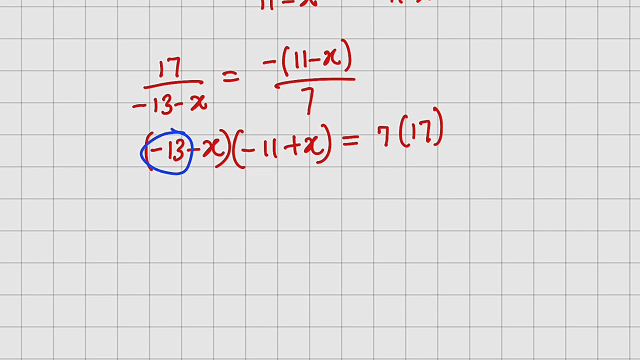 multiplied by negative: 13 minus x, 11 plus x. if you distribute negative inside, This must be equal to 7 multiplied by 17.. Now let us distribute this. We have negative 13 multiplied by negative 11.. Negative negative is positive. Then 13 times 11 is 143.. 143.. Then this multiplied by this will give us negative. 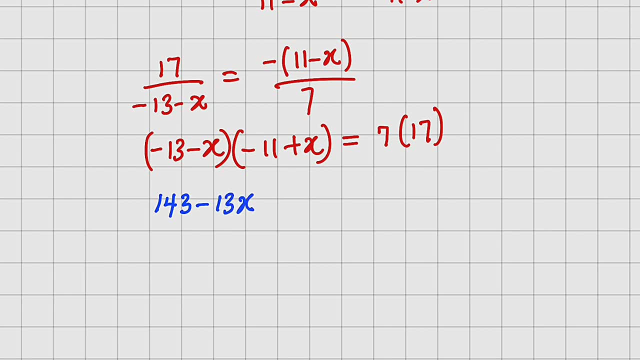 13x, Negative 13x. Then we have negative x multiplied by negative 11.. Negative negative is positive, So we have positive 11x, Then negative positive is negative x times x is x squared, And this is equal to: if you multiply 7 by 17,, you are going to have 119.. These are like. 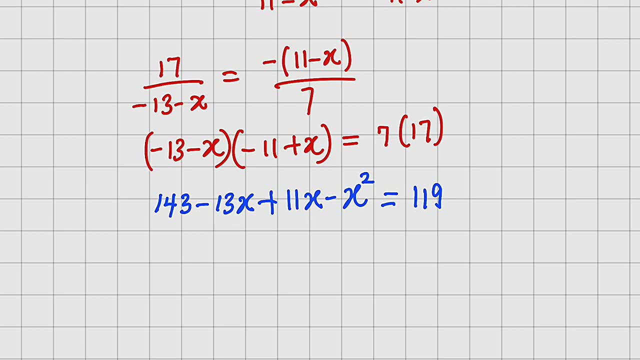 times. If you add them together, you will get 119.. So this, multiplied by 7, multiplied by 17, is negative 11x. So we have 143 minus 2x, Then minus x squared, And this is equal to 119..